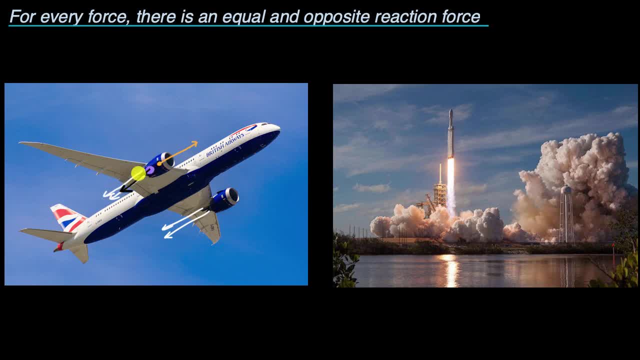 By pushing on these particles and accelerating them backward by exerting a force on them. the equal and opposite force is the force that the particles, those molecules of air are exerting on the jet and moving it forward. The same thing here is going on with this rocket. 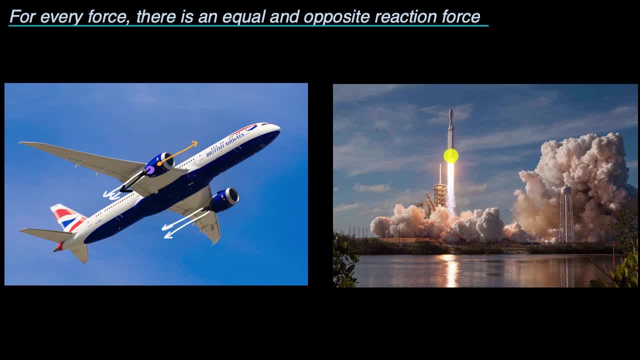 You have some rocket fuel in there. It gets ignited, it explodes, And as it explodes, there's a force that exerts on those little molecules And that force is going in this direction, But as it does that, there's an equal and opposite force. 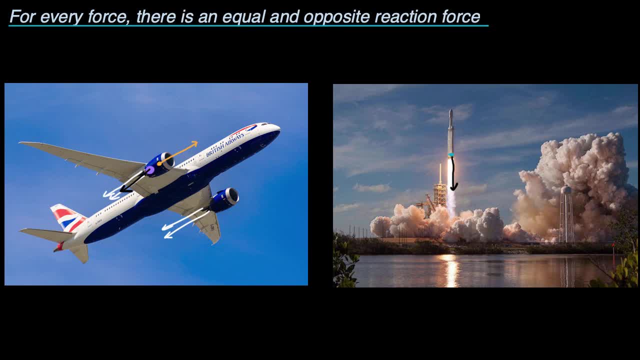 that the molecules are exerting on the rocket. The rocket is having a force acted on it, Once again equal and opposite. So it's important to realize that the reaction force is not on the same object, It's on the other object. 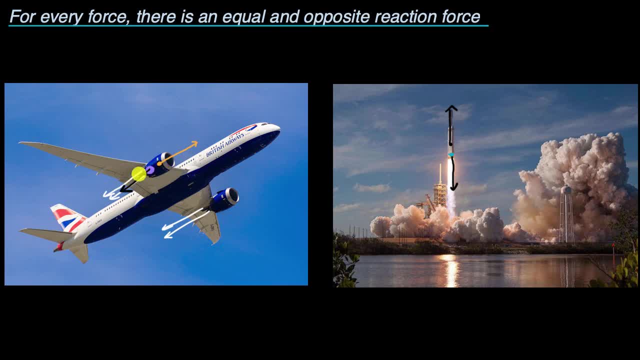 If one object is putting an action force on another, then the second object is putting a reaction force on the first. The forces do not cancel out. It's also important to realize that both forces are generated in pairs and happen at the exact same time. 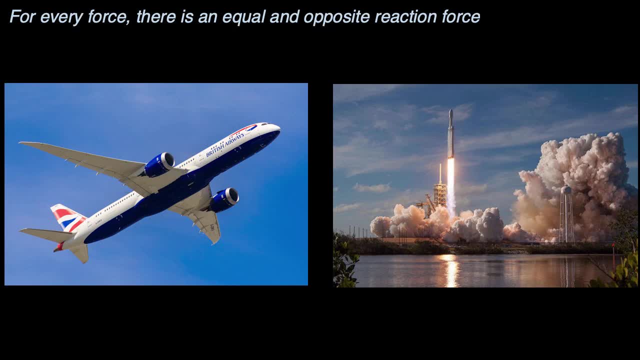 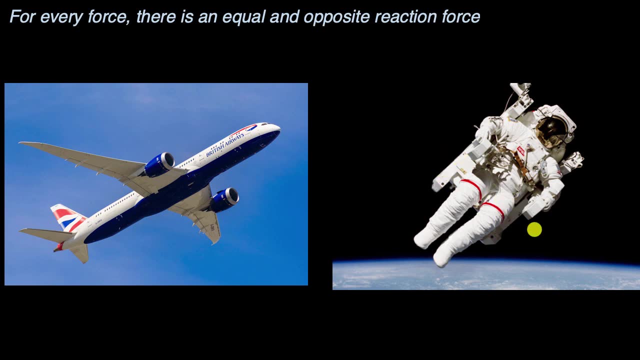 There's no delay. We can look at other examples of this. This is a scenario that I would never want to be caught in being drifting through space. Now this astronaut here has some type of a rocket pack that might help it move around. 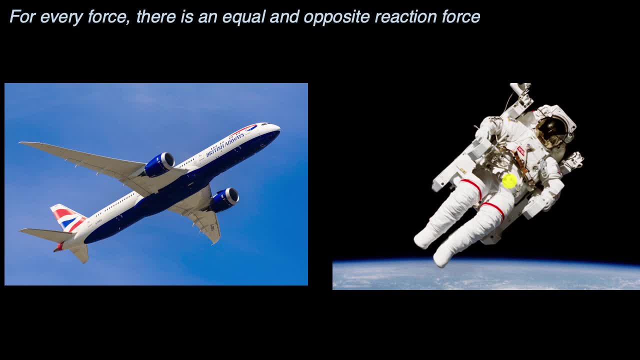 But let's say your rocket pack ran out of fuel and you're just drifting through space. How can you get back to your spaceship? Well, if you have a wrench or something on you that you can throw, if you can take that wrench. 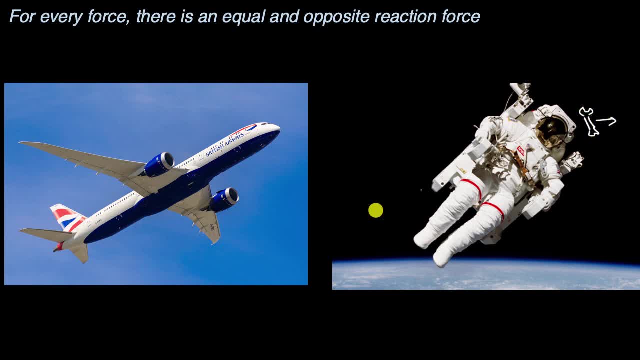 and if you can push that wrench in that direction- and let's say your spaceship is over here to the left- well, the equal and opposite force is the force that the wrench is going to exert on you, the astronaut, and then it will push you in that direction. 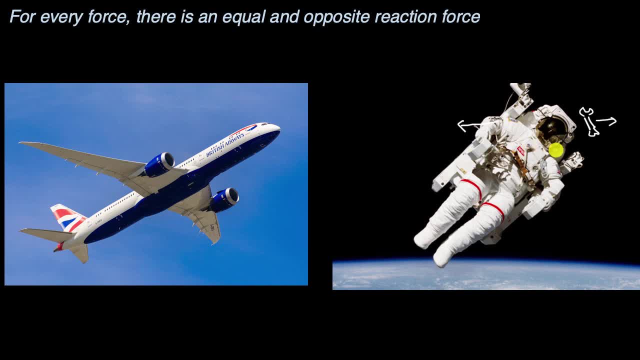 and accelerate you in that direction. So that's a useful thing if you ever get caught drifting through space. but you could do an experiment right now: Press on the table in front of you. When you press on that table, you're clearly putting a force onto that table.